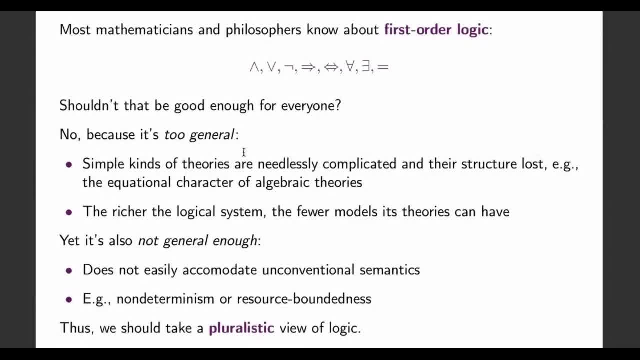 One reason is that in many settings it's too general for its own good, So that you know if you have certain kinds of theories that have a more kind of constrained structure. for example, the algebraic theories are equational in nature. 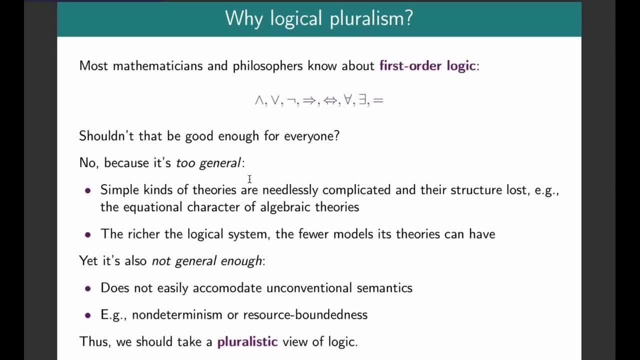 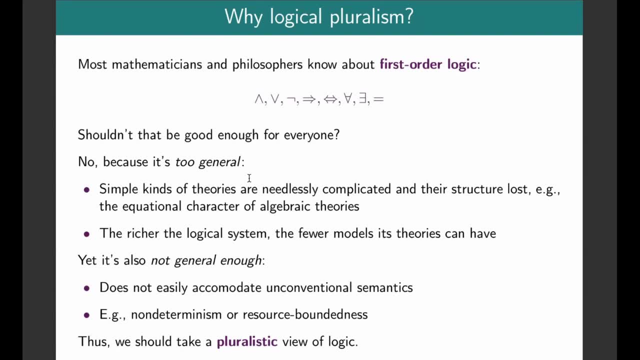 Then this structure is sort of obscured by the formalism of first order logic. But there's a more important reason than this too, that it's too general, which is that it's not, And that is that the richer your logical system is, the fewer kinds of semantics that you can assign to it. 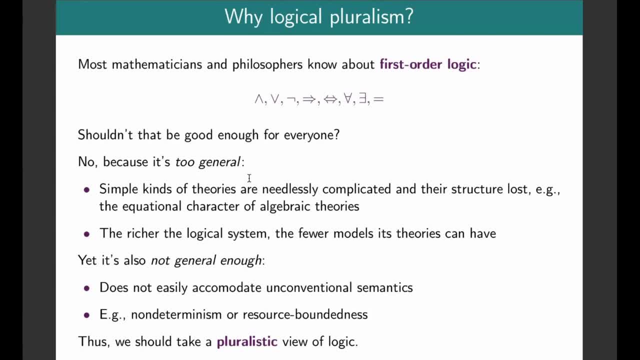 So the fewer types of models you can have for its theories- And we'll see very concretely this idea later. But yet for all that, it also manages to not be general enough for certain purposes, So it doesn't easily accommodate unconventional semantics. 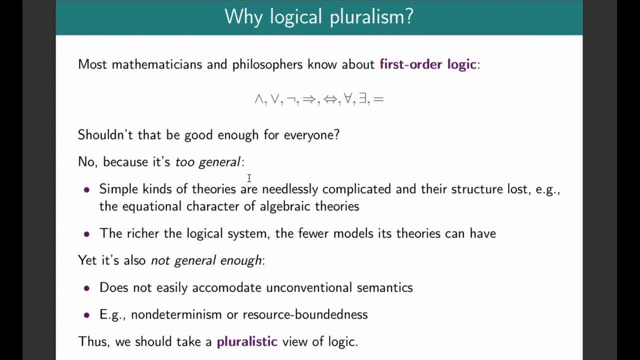 So, for example, one thing which I hope to get to at the end if there's time is, you know, non-determinism. Non-determinism are probabilistic aspects. So you know, one can encode probability theory into first order logic by, but first one has to sort of write down a whole lot of the theory of real analysis to even get there. 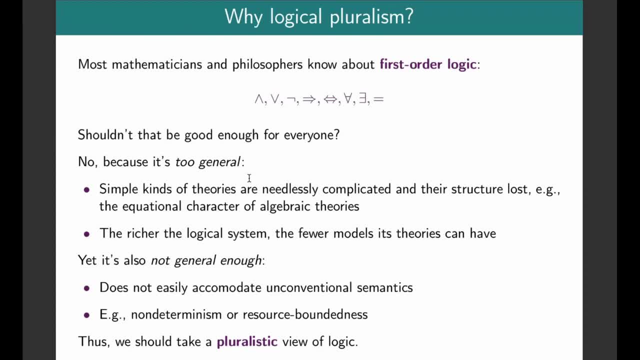 So if you want to have sort of more of a first class view on non-determinism, you want to sort of, if you want to sort of bake that into your logical system, then categorical logic gives you tools to approach that, And so, for all these reasons, I argue that we should take a pluralistic view of logic rather than having one logical system to rule them all. 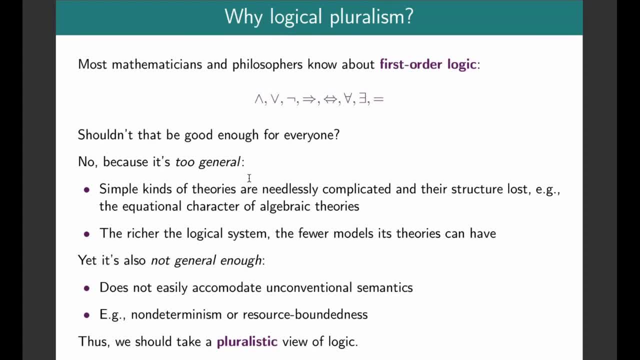 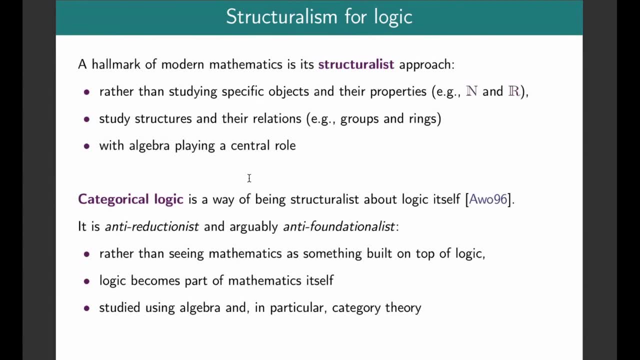 We should have a flexible framework for constructing logical systems, And so how might one go about doing that? I mean, after all, you can always. just you can always. if you think of logical systems is just sets of rules for manipulating symbols. You can always write down some rules. 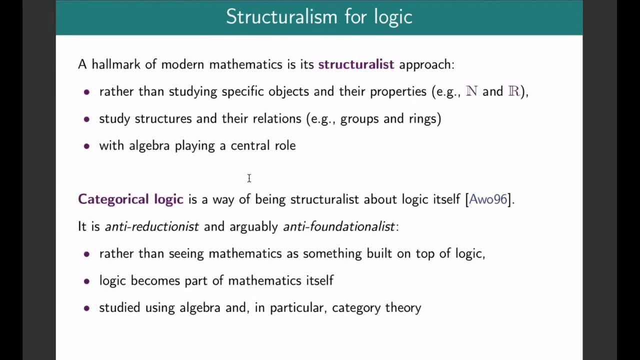 But how do you know whether they're They're any good, or how do you know whether they relate to other systems? And so this is where we can draw on a broad tradition in modern mathematics, which is which is sometimes called mathematical structural structuralism. 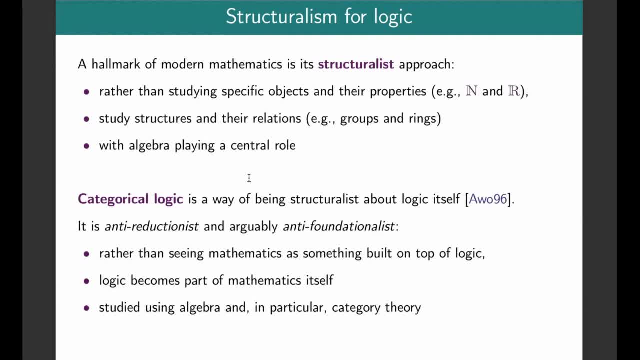 So, rather than studying specific objects in their properties, such as, like the natural numbers or other certain number systems, we're going to study abstract structures, the axiomatized aspects of those systems, And we're going to study the relations of those Structures to each other. 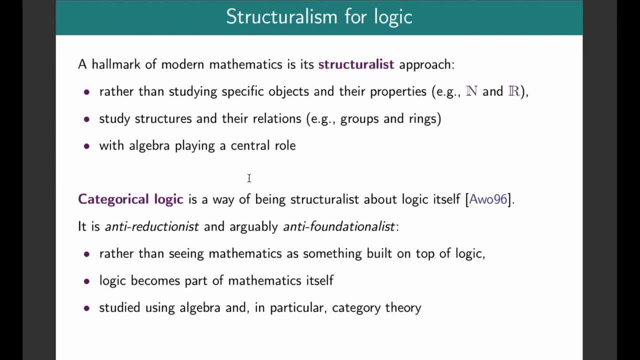 So you know, for example, in classical abstract algebra we would study groups and rings, And algebra has played a central role in this approach to mathematics. And so one way to think about categorical logic is that it's a way of being structuralist about logic itself. 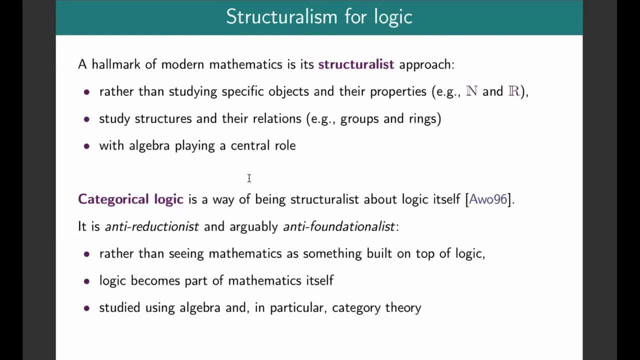 We're going to apply the structuralist philosophy to study logic itself And in this sense I think there's something sort of anti reductionist about categorical logic. So in the traditional conception of the role of logic in mathematics, logic, The logical system is, is at the foundation, and mathematics is this great edifice built on top of it. 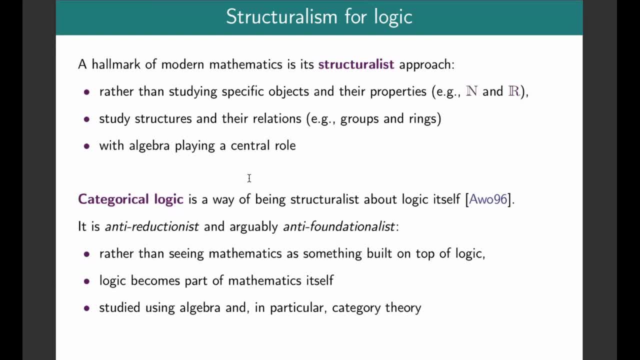 But from we sort of categorical logic sort of turns it on its head a bit, because now we're going to make logic into just a part of mathematics itself. It's not going to have any really special status And we're in and, moreover, we're going to study it using the same methods that we study other things in mathematics. 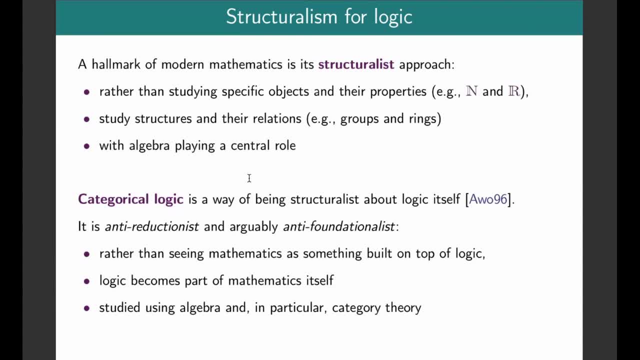 In particular, we're going to use algebra, And within that we're going to use methods of categorization, And that's going to be called categorically theory, OK, so. so there's a lot more that can be be said about these sort of philosophical ideas, but I'll leave it at that. 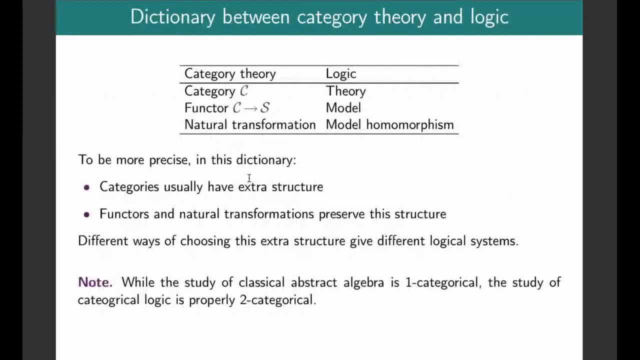 And now I want to try to get into some of the basic ideas here. So here is a to the first approximation. category categorical logic establishes the following dictionary between category theory in logic Right, So to to a rough approximation. It's an algorithm. 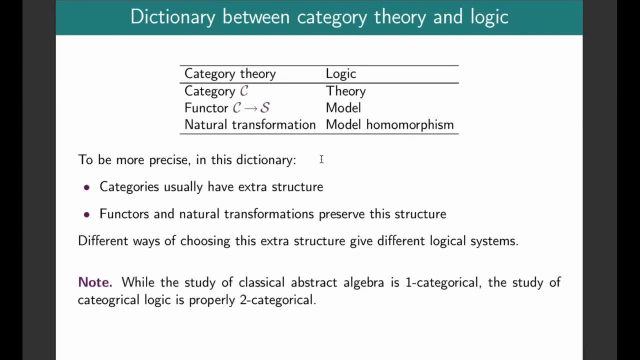 approximation. categorical logic establishes this dictionary. So we're going to think of logical theories as corresponding to small categories and we're going to think of functors out of those categories into some category S, which for now we can just think of as the 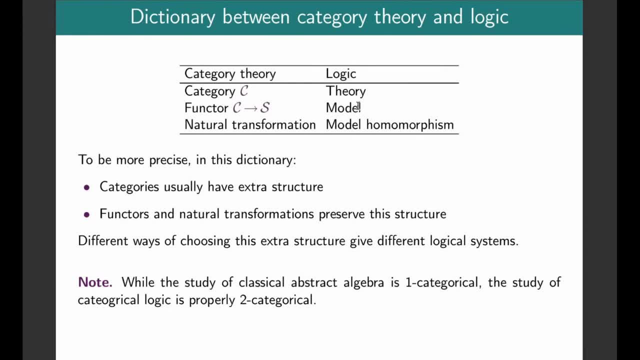 usual category of sets and functions. Those will be models of the theories, and then natural transformations between those functors will play the role of model homomorphisms, And so I'll make this a bit more concrete shortly, But first I should say that this table's 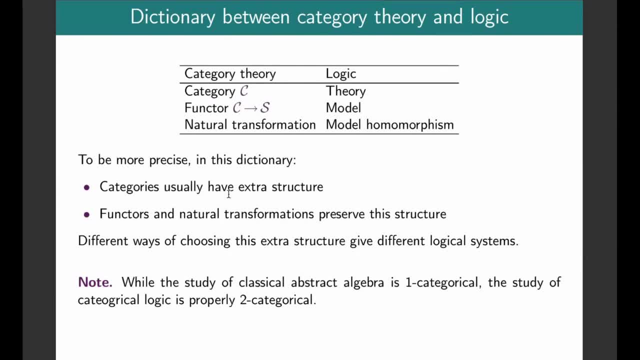 a bit misleading in that usually we're going to want the categories to have some extra structure, And it's precisely this choice of extra structure that will give us different logical systems, So by kind of equipping our categories with various kinds of homomorphisms. 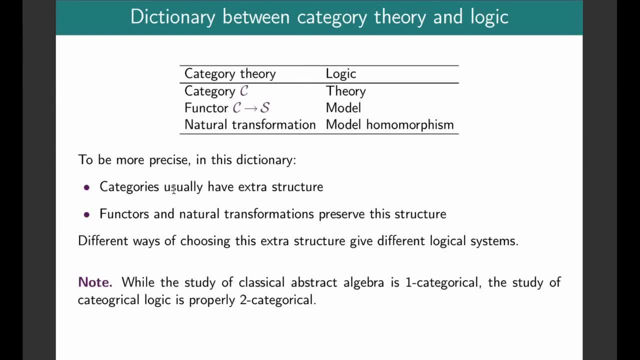 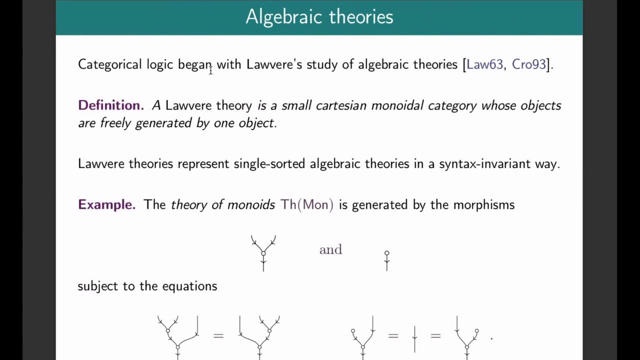 extra gadgets. that was what allowed us to have different logics, And then, once we've done that, we'll want the functors and natural transformations to preserve this additional structure. I'll skip this last remark. Okay, so I'm going to begin with algebraic theories. 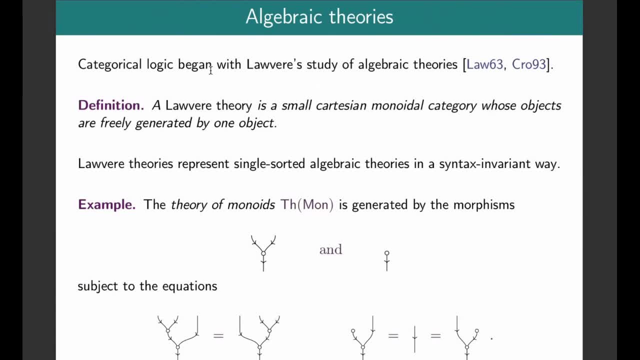 which is appropriate, because that's where categorical logic began with Laver's study of algebraic theories, And so a lot of your theory is a certain kind of category, in this case a Cartesian category, whose objects are freely generated by one distinguished object. And that last 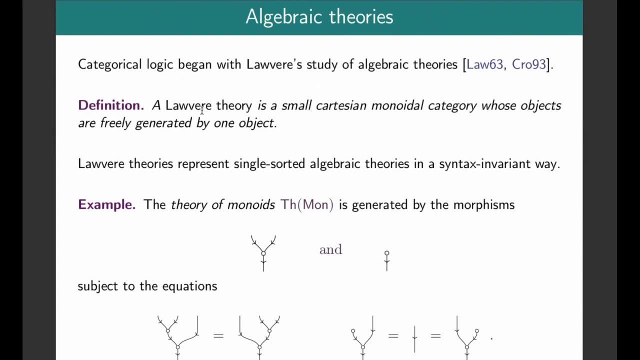 condition sounds a little odd, but the purpose of it is to essentially make this represent a single-sorted algebraic theory. So, to give an example of this, the theory of monoids is going to be a Cartesian category which is generated by two morphisms. 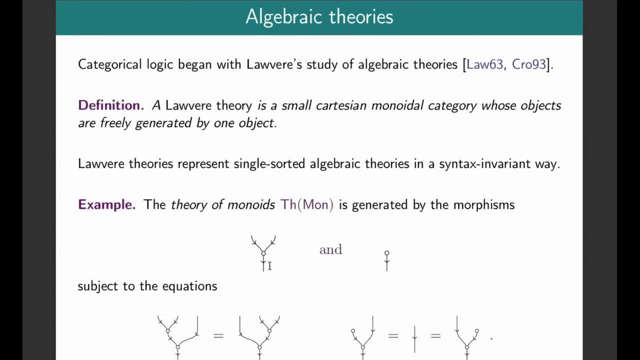 that look like this. So these are drawing these as string diagrams so you read them from top to bottom. So this first one is like the monoid multiplication: It has two inputs and one output. And the second one is the monoid unit and it has a single output And 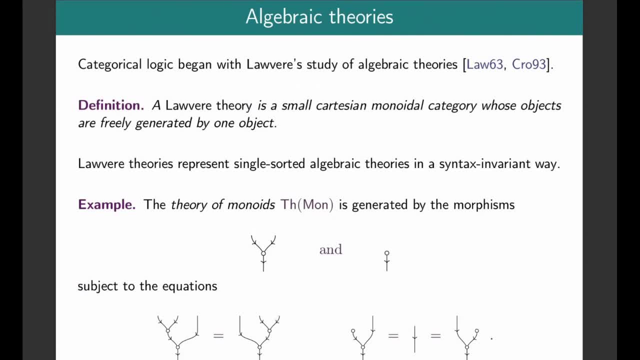 then it's subject to these equations, which the first one is associativity And then the second one is unitality, And the point I want to make here is that a lot of your theories represent single-sorted algebraic theories in a syntax invariant way. So you know I'm 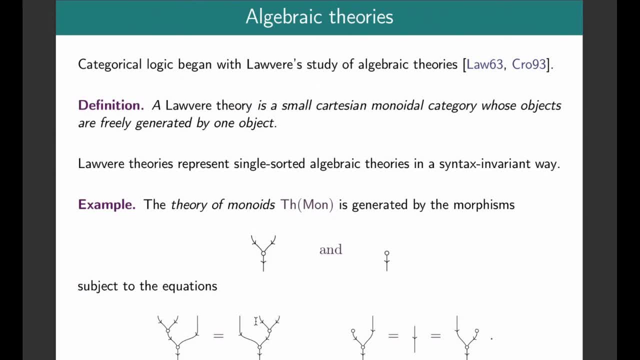 drawing these using string diagrams. I could also draw them using just like regular symbols, and that would represent the same thing. So this is already a departure from conventional logic, where logical theories are fundamental, Generally syntactical objects. that is not quite the case anymore, And we'll see more. 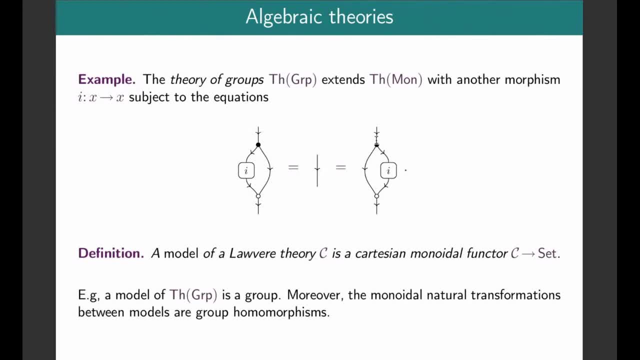 about this idea, but first I want to give one more example. So the theory of groups, basically, is what you get by taking this theory of monoids and adding some another, another, generating morphism. this, this thing, I, which is supposed to represent the inverse operation. 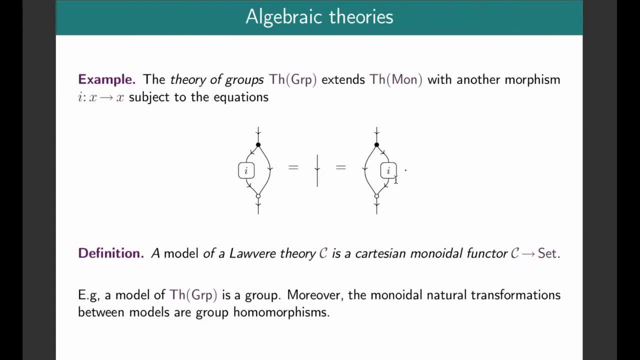 in the group. And then these two equations assocering that, you know, this thing acts as a left operator. this Joe, So the right operator, you know, has essentially given to write inverse on every element. And so this black thing at the top of the diagram, 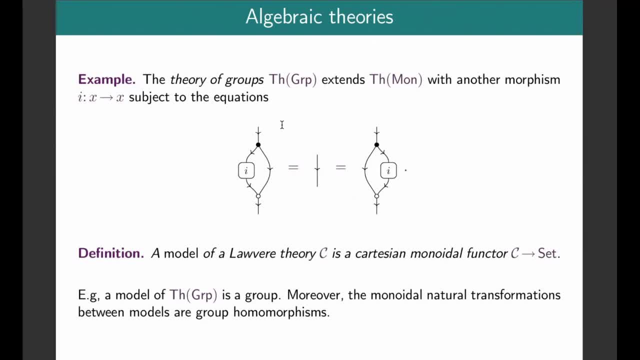 is representing the operation of copying, So it's copying the input and then applying the inverse to it in the identity and then checking that once you apply the multiplication, you get back the original element. Okay, And so, in accordance with the general dictionary, 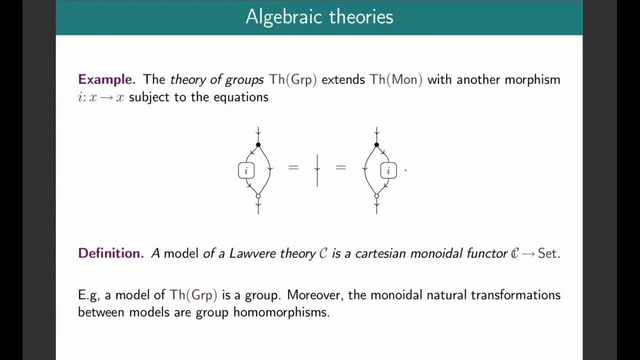 a model of a logger theory will be a Cartesian functor out of this category C into the category of sets and functions. And so, as you would expect, a model of the theory of groups is indeed a group And, moreover, the monoidal natural transformations between these models. 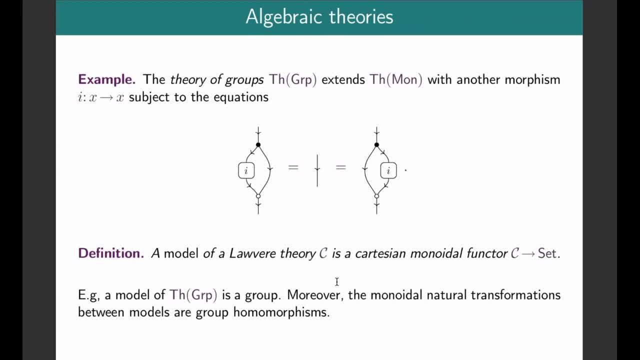 are the group homomorphisms. So this is just a sanity check that this is reproducing the right thing. Evan, can I interrupt? I think there's a typo on this, because shouldn't the middle thing be Yeah? Like it stops and then puts out the identity element every time. 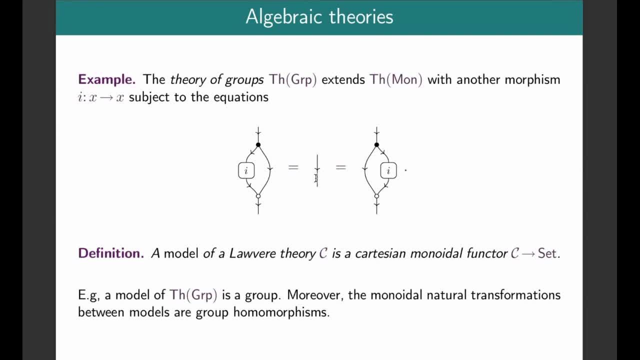 The middle thing, The middle, Yeah. Shouldn't that be like a black dot, stopping it, and then like a unit? No, because this is the law, that Isn't this. A times A inverse is: E Is the identity. Oh, good point, Let's see. 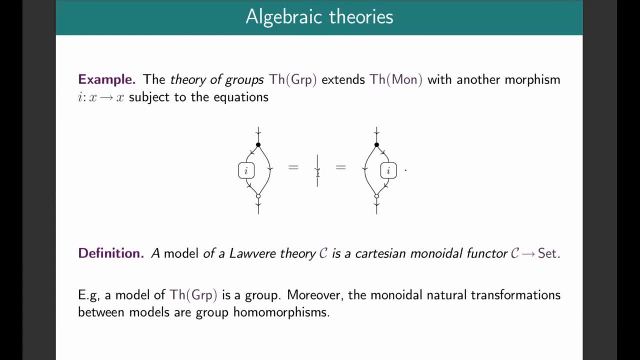 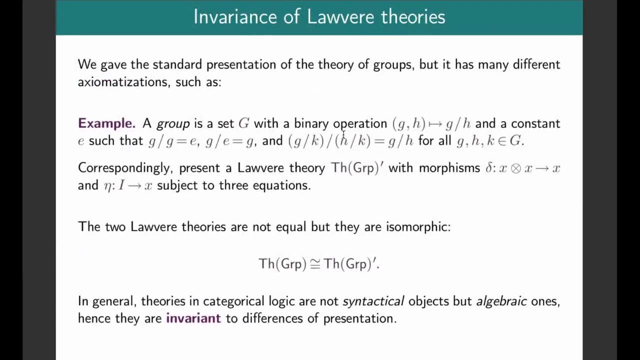 You're right. Yeah, sorry, that's a typo. Sorry about that. I'll fix that in the slides. Thank you, David. Okay, We've seen one way in which logger theories are sort of invariant, but there's a deeper sense of this, so let's explain that. 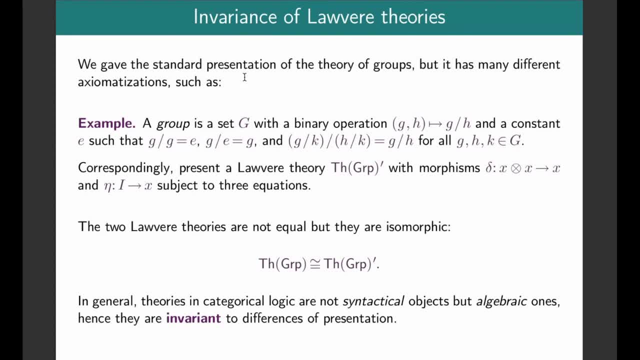 Thanks. what I just gave modulo, that typo, is the sort of standard presentation of the theory of groups, but actually there are lots of different equivalent ways to axiomatize a group. that may be less familiar, but some of them are actually kind of interesting. so here's one where we one one turns out. an equivalent way to define a group is as a set. 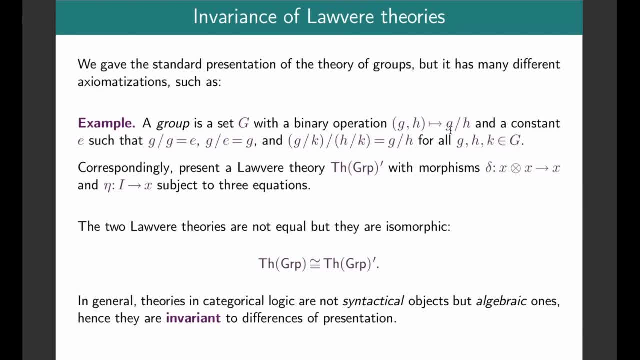 equipped with a binary operation, which represents division and a constant e satisfying some equations, and so we interpret this as, like: g divided by h is supposed to be g times h inverse, and so we could write down: you know a lot of your theory that is presented by you know morphisms. 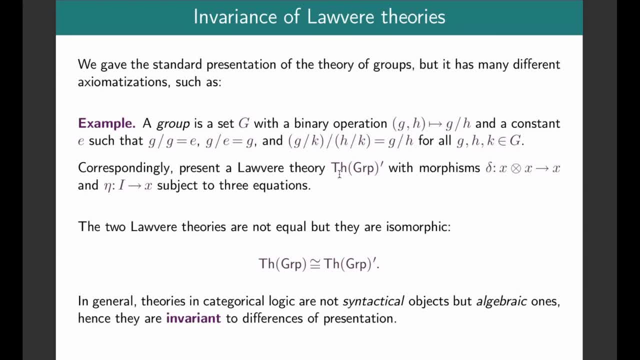 corresponding to these operations and subject to the three corresponding equations, and that will give me another category and these, you know, morphisms corresponding to these operations, and that will give me another category. and these categories aren't equal, um, but but they are isomorphic. and the and the isomorphism between 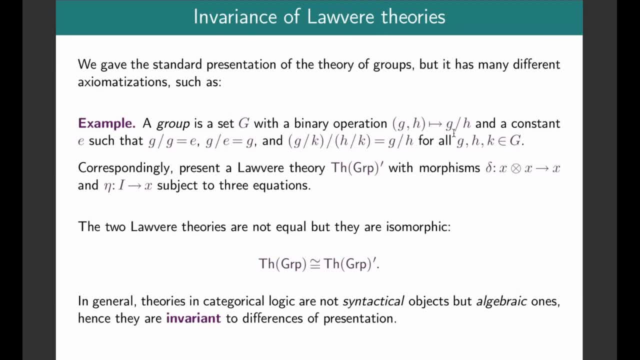 them, um is what's going to basically map these operations in one, into the corresponding thing, and together um, and and so the. the point here is that theories and categorical logic are not um, they're not syntactical things, they're, they're algebraic ones and hence they're invariants. 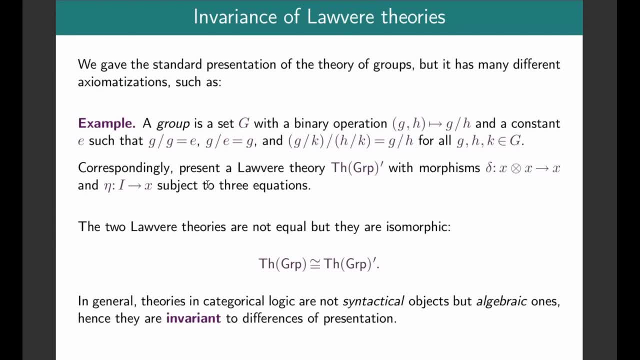 invariant to differences of presentation. so note the level shift involved here. right, so you, if you've learned, you know about, you know groups and abstract algebra. you learned that you know there are different ways of presenting a group, but they both all define the same mathematical object, up to isomorphism. well, here you know, the theory of groups is now being 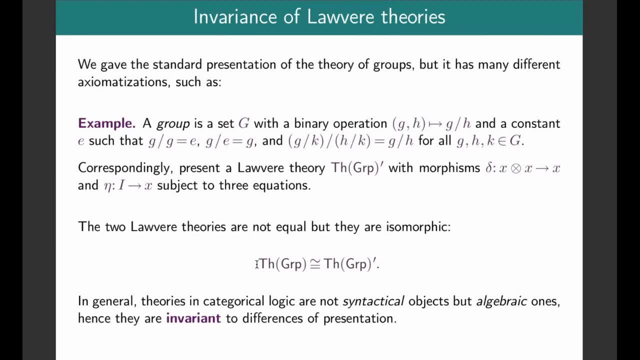 presented by generators and relations effectively, in different ways of presenting it, gives rise to the same mathematical object. i'm confused by this notation. should the prime be on the inside of the parentheses on the right side? yeah, the notation's a little loose there, um, because i'm i'm. 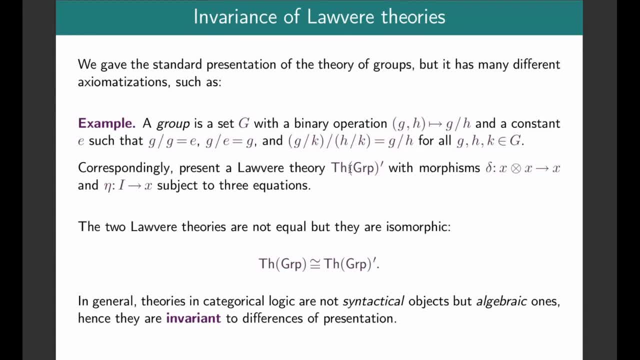 i'm sort of writing theory of groups as if this theory, as if are you changing the theory functor or are you changing the? yeah, so what i'm saying here is that you should just think of, rather than thinking of this as a mapping from the category groups to some kind of theory, just oh, erp is the. 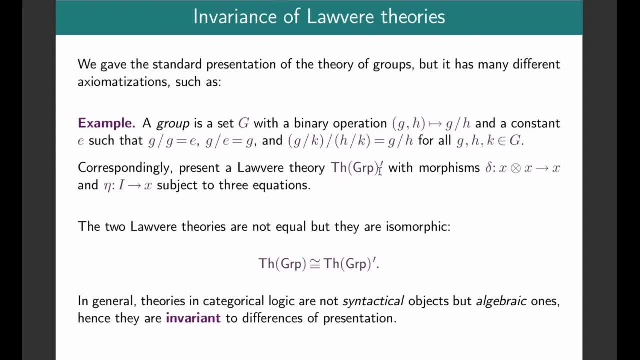 category group and not a representation. okay, yeah, so. so just think of both. yeah, so don't read. yeah, that notation is a little. is there a variable here for the presentation itself? uh, no, so, yeah, so. so this, the theory, this theory groups, just represents the, the law of your theory. 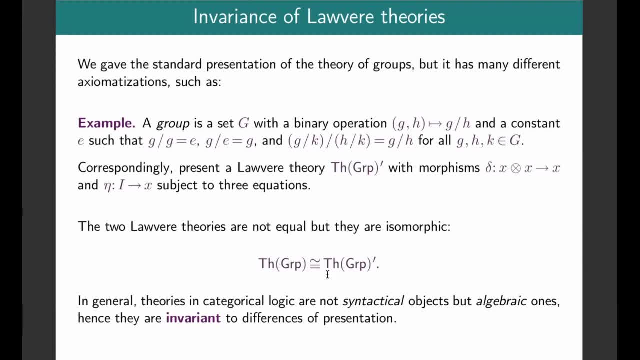 their cartesian category presented by those things, and so, um, and the prime here is the one corresponding to this other way of axiomatizing it. okay, so you could instead of said: there's some theory, operation, and then you've got two different presentations and the theory of the first. 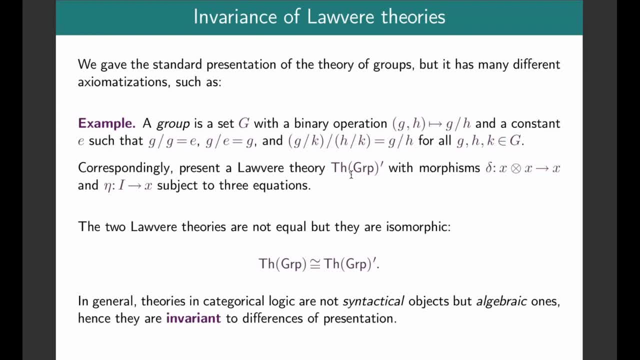 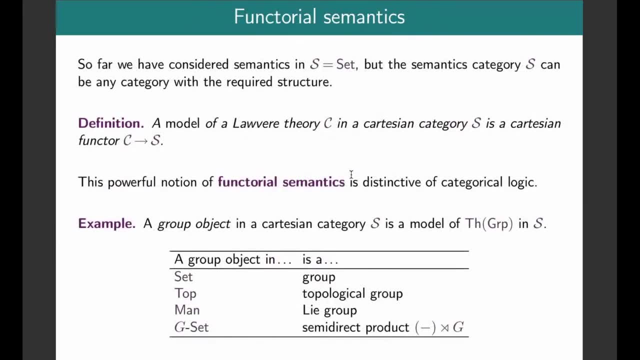 presentation is isomorphic to the theory of the second presentation. yeah, i could have said okay, okay, so. so now we come to another powerful aspect of of categorical logic, which is the idea of functorial semantics. so so far we've been considering semantics in this category. uh, 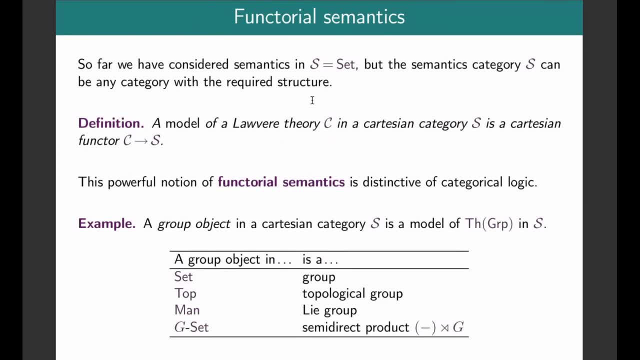 on the category of sets and functions, which is certainly sort of the default setup. but the semantics category can be placed with any category that has the needed structure. so in the case of logger theories we can say that if i give you any cartesian category s, i can say that a model of a logger 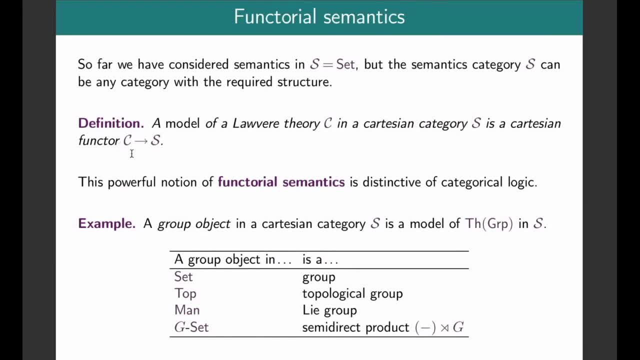 theory in that category is just a cartesian functor from c to s, and this is a pretty distinctive feature of categorical logic and it allows you to interpret theories in other kinds of settings. so here's sort of some classic examples like you can say that a group object 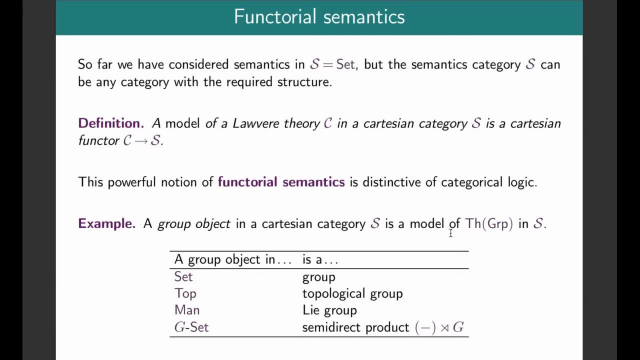 is going to be in a particular cartesian category, so going to be a model of the theory of groups in that category. and you know, so we've seen that a group, object and set is of course a group. and you can also recover some other famous mathematical concepts by just saying: oh wait, what's a group? 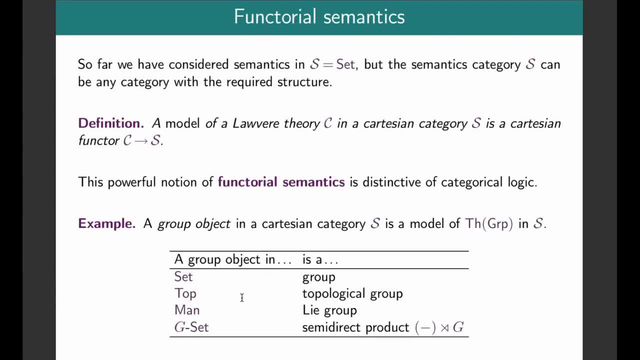 object in this category. so a group object in category of topological spaces, a topological group, a group object in the category of smooth manifolds is a lee group. turns out that you unpack what's going on. A group object in the category of group actions by some fixed group G. 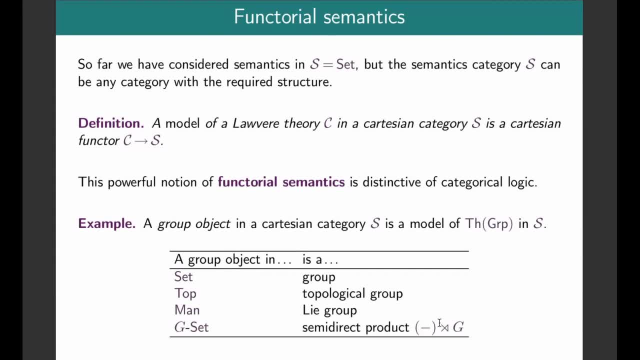 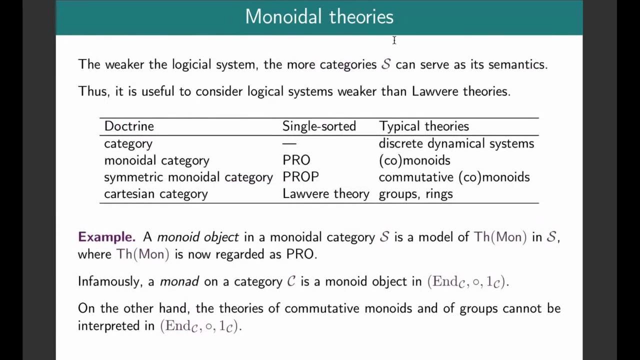 turns out to be a group, that is a semi-direct product by G. So it's a favorite hobby of category theorists, to you know. look for group objects and monoid objects, as we'll see in various places, and see what you get. So, having arrived at this point of view, though, 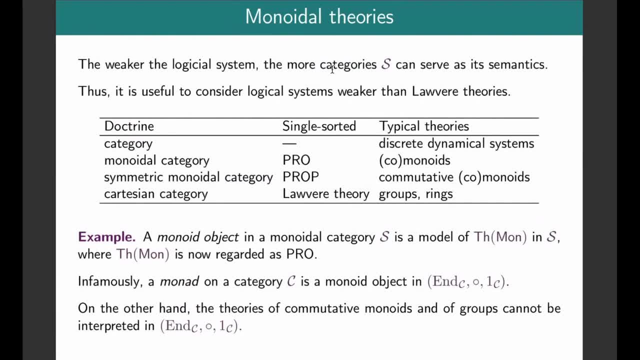 we can start to understand why it's useful to not have a single logical system but to have ones that are also weaker, Because the less structure your logical system has, the more categories S you can choose to take semantics in, And this is a very powerful thing. 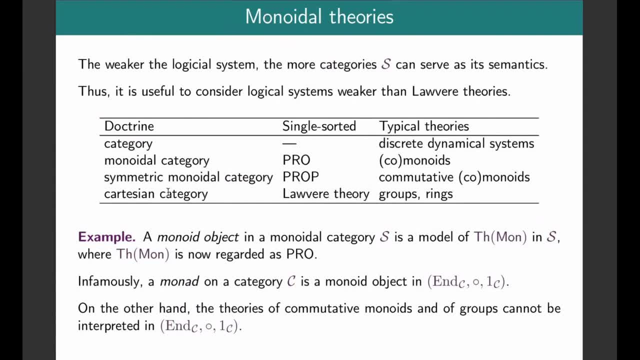 So you know we've been considering lobbyer theories. These are Cartesian monodal categories and what's shown above here are some successive sort of weakenings of the structure involved. So we can look at various kinds of what are some of the things called like monoidal theories. in the single sorted case they correspond to these things called props and pros. 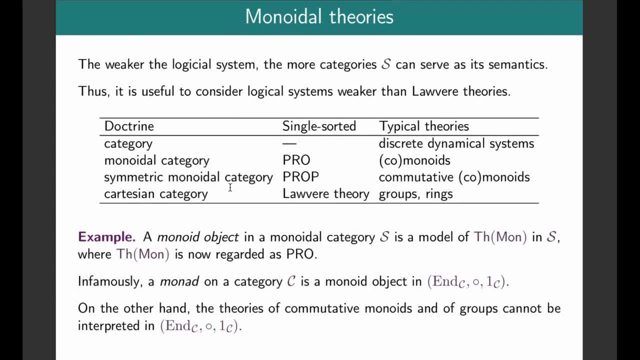 But the, and so I won't fully unpack this table because there's a lot going on here. But what I will say is that we saw previously the theory of monoids and it turns out that, you know, we don't actually need the full structure of a lobbyer theory to express that. 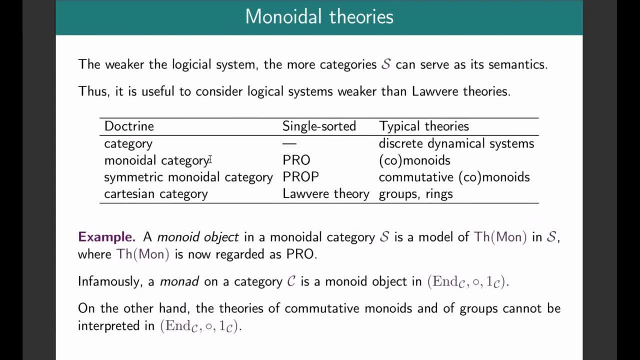 We can express the theory of monoids in any pro, And an advantage of this is that we can look at models of the theory of monoids, called monoid objects, in any old monodal category. So I couldn't resist putting this in here. 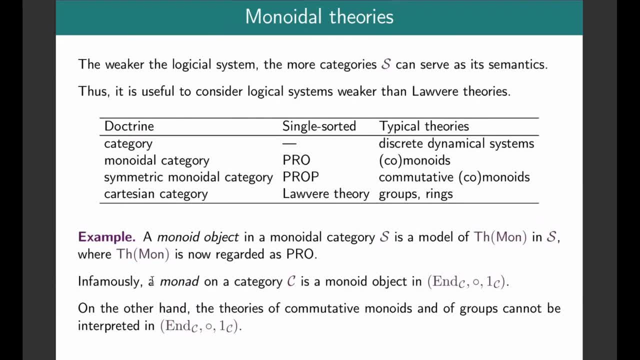 So it's sort of a notorious joke about category theory that all a monad on a category is a monoid in this category of endofunctors. Well, that is a true statement, but it's also just an instance of this principle of composure. 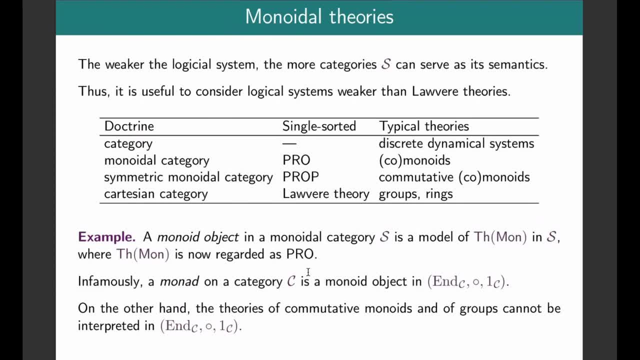 of functorial semantics And I want to make the point that I'm not terribly interested in monads in this talk. but what I do want to make is the point that the theories of commutative monoids can't be expressed in this category, because this category of endofunctors 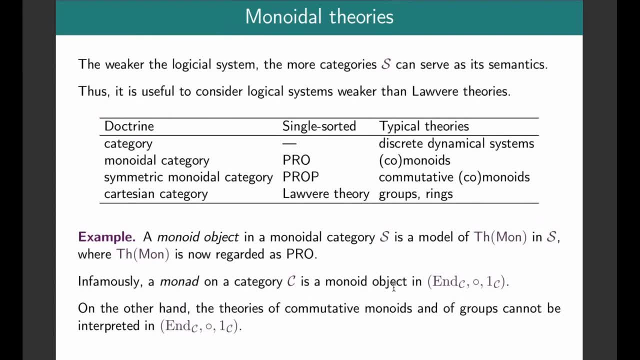 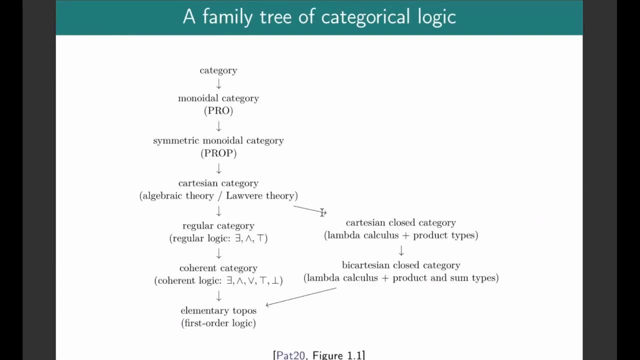 isn't symmetric monoidal. So this really shows why it's useful to be able to fit logical theories into the weakest system that can accommodate them. Okay, So to zoom out a little bit, here's what you might call a family tree of some. 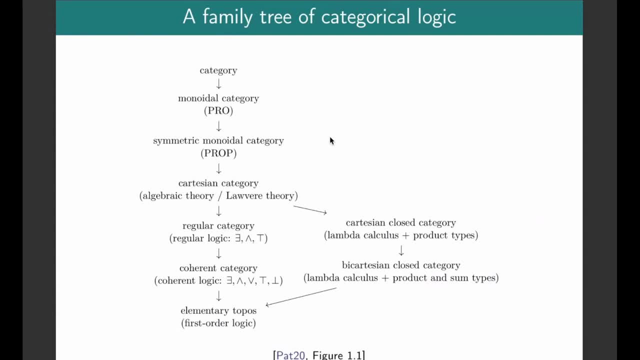 of the most studied parts of categorical logic. So I just want to include this to give you a flavor. So we sort of seen that. So subject began with algebraic theories, with law of your theories, and we've seen that you can. 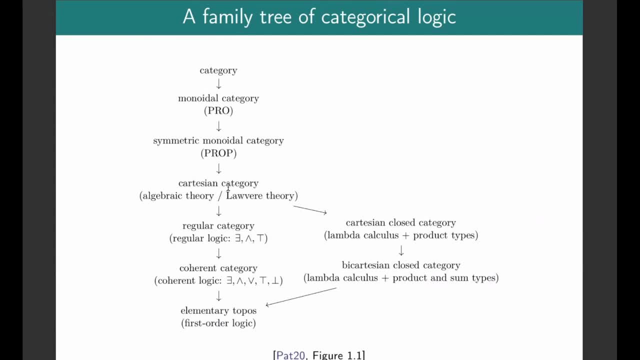 successfully remove structure and that there's value in doing that. You can also sort of successively add structure. So there's sort of a progression from Cartesian categories to regular categories, which corresponds to a fragment of first-order logic called regular logic, on to coherent logic and finally to elementary toposes, which are formalizing. 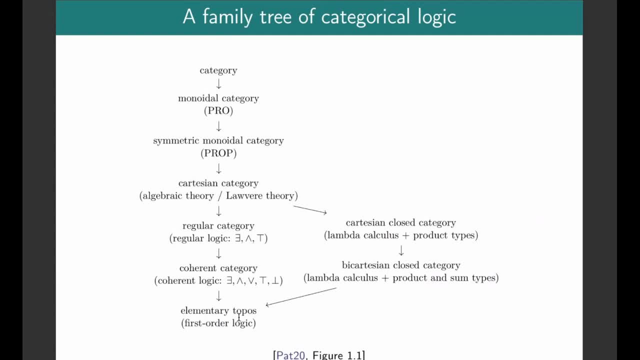 basically a kind of intuitionistic first-order logic. And there's also a sort of branch of the family tree here which is more traditionally associated with computer science, involving lambda calculus and Cartesian closed categories. So I'm not going to get into this here. but 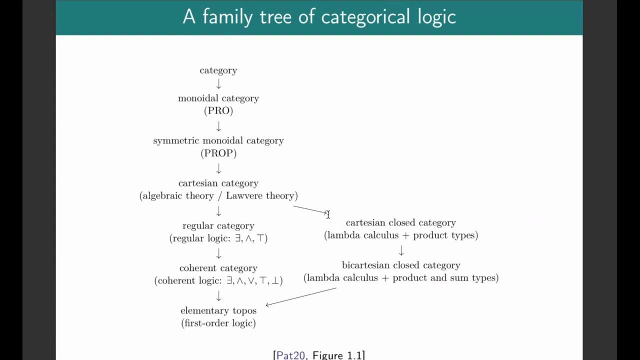 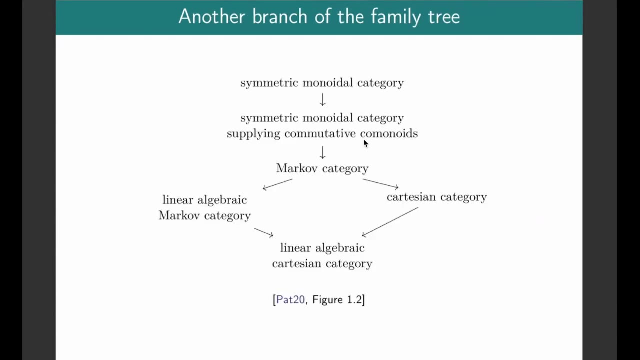 this is a bit useful to have. This is sort of a layup of some of the land. How am I doing on time? You're doing okay. We're near the end, but don't feel too rushed Okay, so I'll wrap up pretty soon. So, just to conclude, I want to 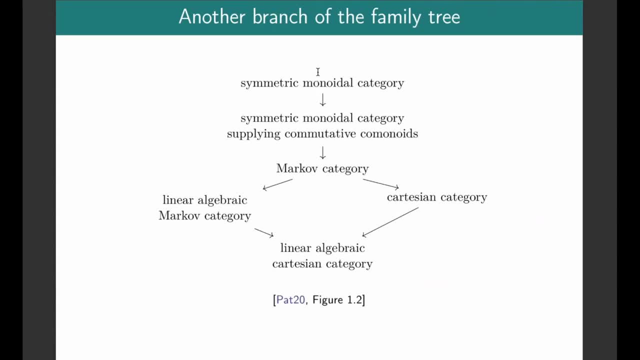 kind of explore a more non-conventional branch of the family tree. So this is kind of getting closer to things that I've worked on myself, And so this is the idea of the family tree, of a weakening of Cartesian categories to these things called Markov categories. 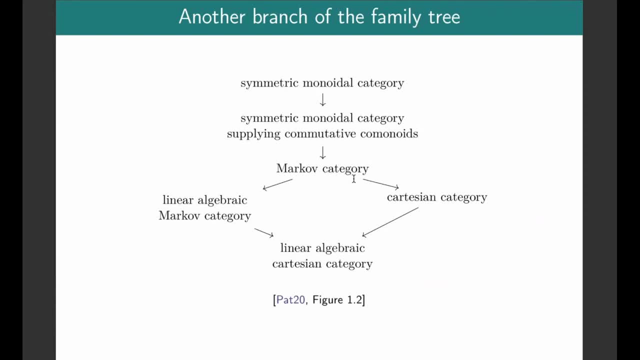 which I believe Toby already mentioned in his talk, And this will allow us to accommodate non-determinism in a way that doesn't really fit into the lobbyer theories and their more expressive systems very well. So the objective here is to try to upgrade our dictionary. 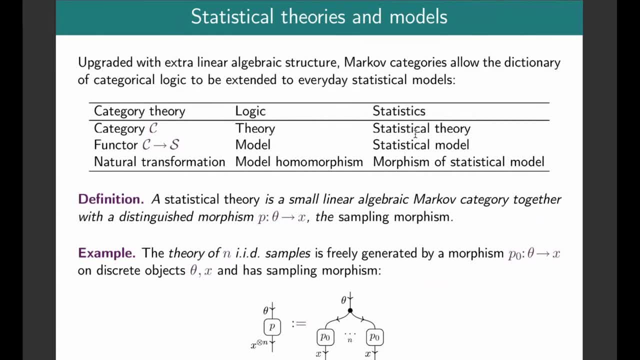 to include also some ideas from statistics now. So there's actually quite a tradition in the philosophy of science and statistics of thinking of statistical models as being somehow actually related to the idea of models and logic. but the purpose of this is to actually try is to try to make that precise. 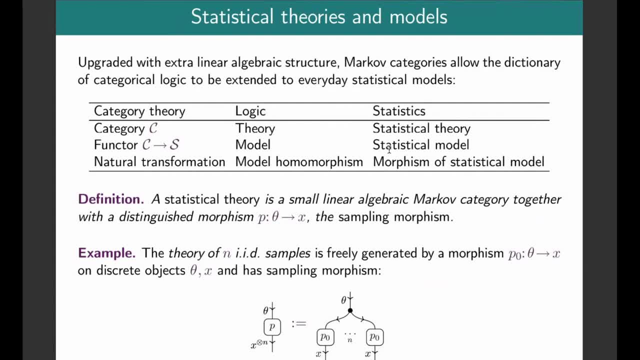 and put some mathematical meat on that idea, And so we're going to so these Markov categories. I feel like sort of feel like I'm missing a slide, but the idea here is that a Markov category weakens the copying axiom in a Cartesian category. 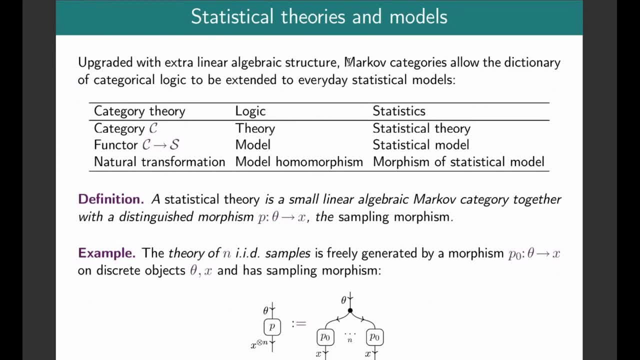 to accommodate non-determinism, And at this point I'm just giving a very sort of a broad sketch. but the idea here is that within this logical system, when you upgrade it further with some linear algebraic ideas which are needed to talk about a lot of. 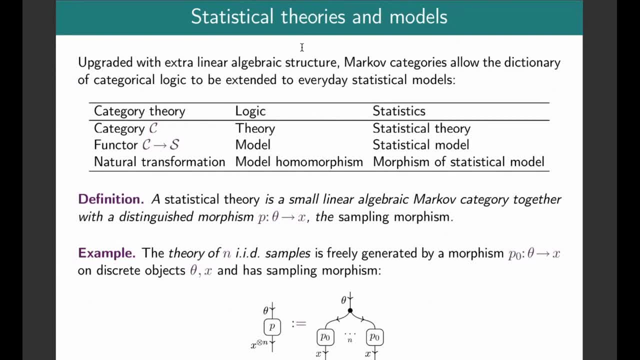 kind of everyday statistical models. you can start to express a variety of common statistical models within this sort of framework. So here's a simple one. at the bottom is the theory of what you might call IID samples. So any statistical model which you get.